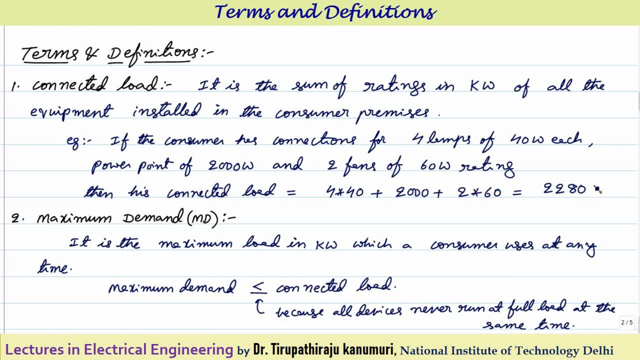 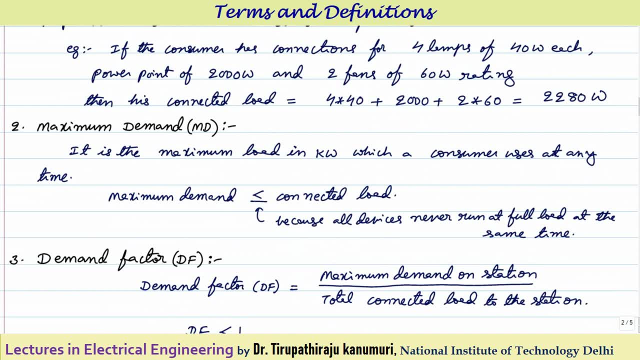 I will consume double 280 watts. So this is called as the connected load. So now all these load are simultaneously never switched on for most of the cases, because we will simultaneously use only some part of the equipment, Like if you take, for example, in your home, also you will have may have. 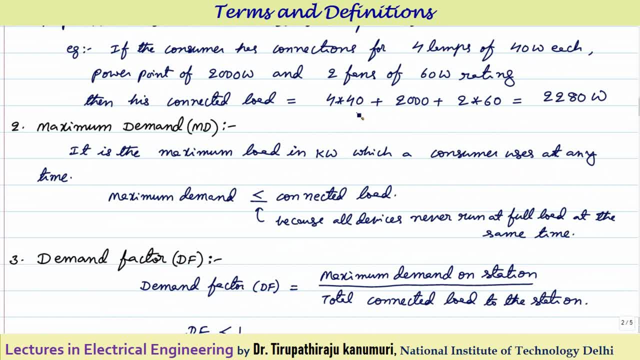 the microwave, oven, washing machine, geyser, So all are not used simultaneously. So that's why, in practice, that demand or that amount of the units consumed from your system will not be equal to the connected load. It will always be less than the connected load. 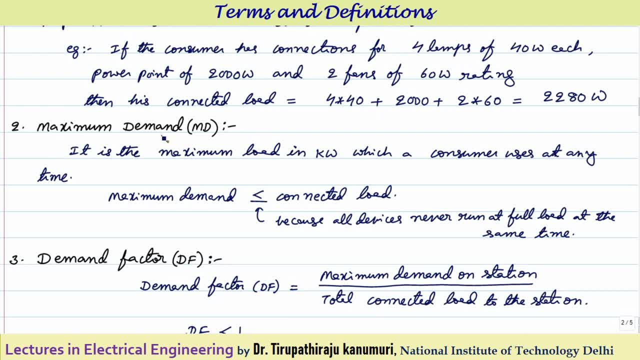 That is given by the term called as maximum demand. So maximum demand means it is the maximum load in kilowatt which a consumer uses at any time. So it is the maximum load in kilowatt which a consumer uses at any time. I told you that practically all the loads are not connected. 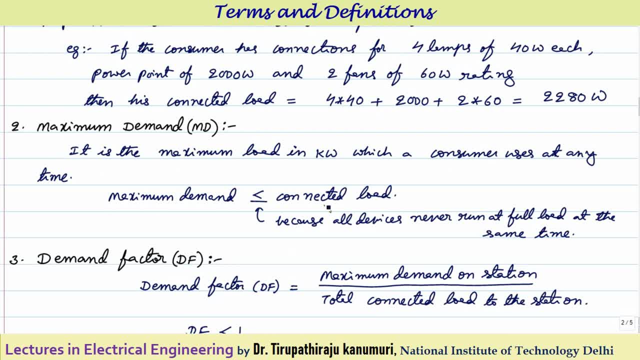 simultaneously. So that is why, in practice, that demand or that amount of the units consumed from your system will not be equal to the connected load. It will always be less than the connected load. That's why, always, the maximum demand will be less than the connected load. This is for concern to the consumer. 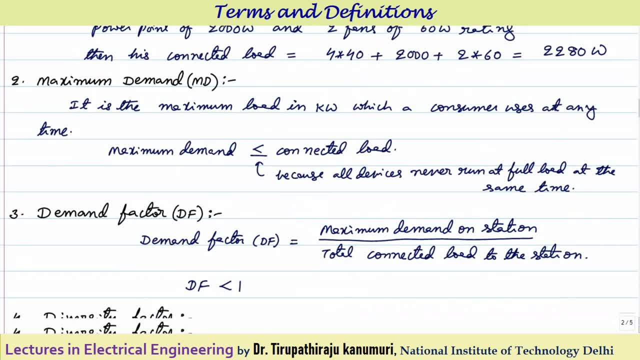 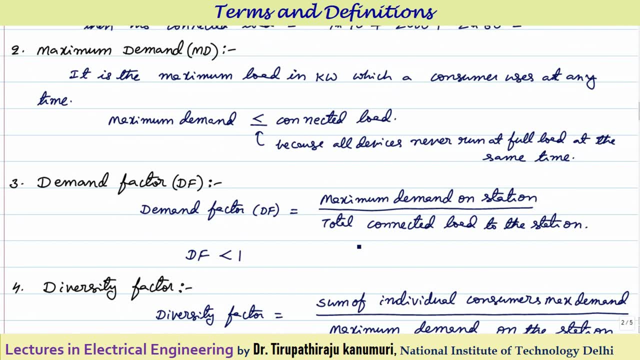 So similar way we can calculate the maximum demand on the power station also. So when you take a power station, many houses or many loads are connected to the power station. So the sum of all the connected loads- that gives the connected load of your power station and maximum demand, means how much is the. 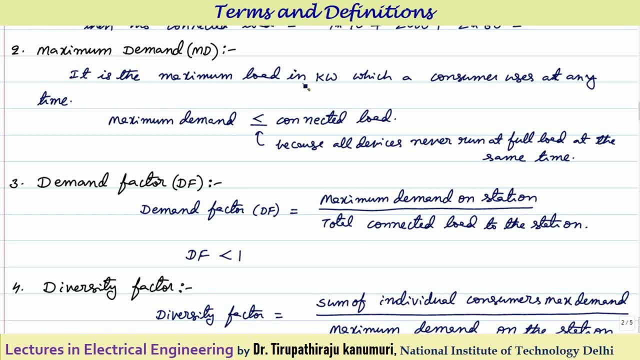 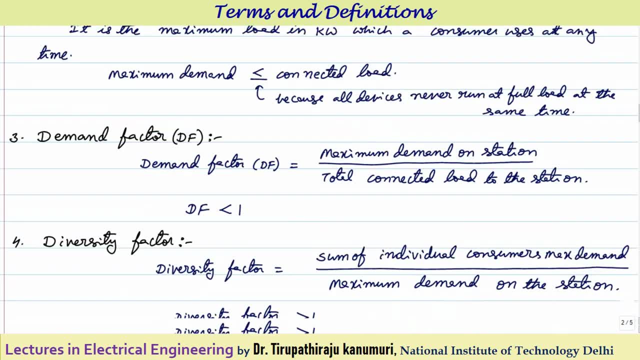 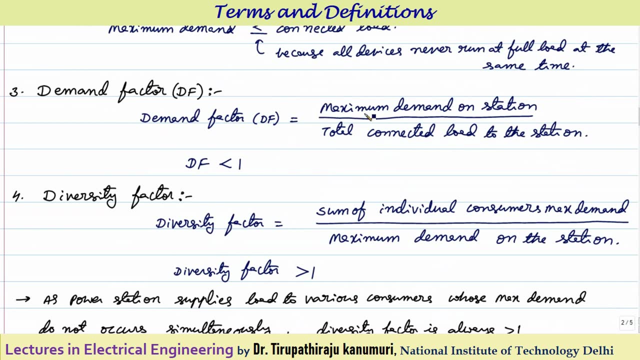 at any particular instant, what is the maximum load that is supplied by your power plant? So that is given by the maximum demand of your power plant. So there comes a factor called as demand factor. The term is demand factor. Demand factor is a ratio of maximum demand on the station divided by. 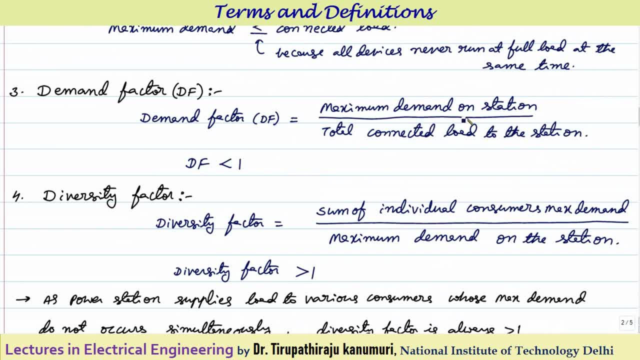 total connected load on the station, Because practically- let us take, for example, I am taking a substation- On the substation, let us assume 10 houses are connected, So in this 10 houses what each house will have some connected load. So the term of the total connected load. 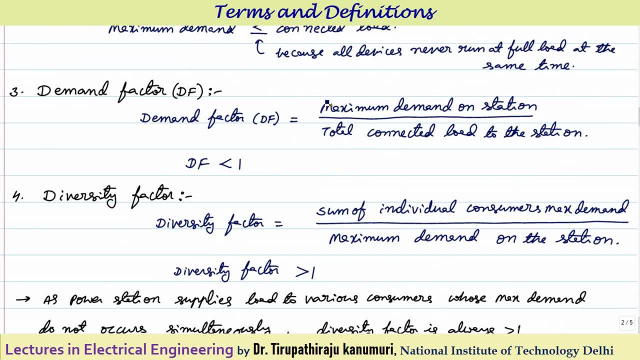 that gives the total connected load on that substation But at a simultaneously. all the loads are not switched on by all the consumers. Different consumer will have the different maximum demand at different times. So simultaneous maximum demand on the station will be always less than the connected load. 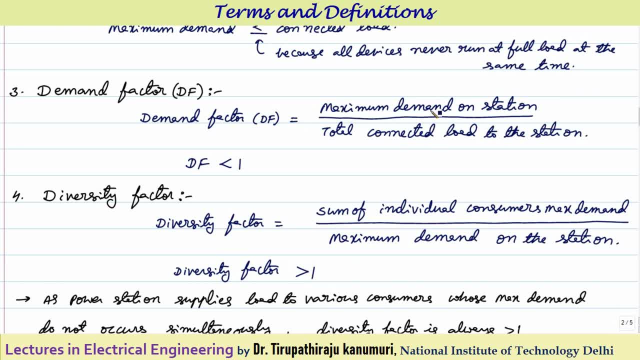 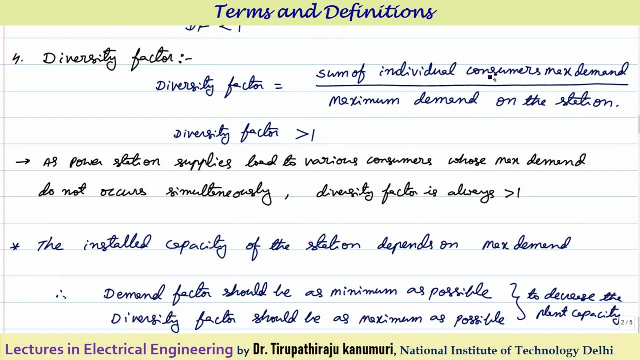 So that is given by the demand factor. That means demand factor is a ratio of maximum demand on the station divided by total connected load to the station. So always this factor will be less than 1.. So then comes the diversity factor. The diversity factor is the sum of individual consumers, maximum demand divided by 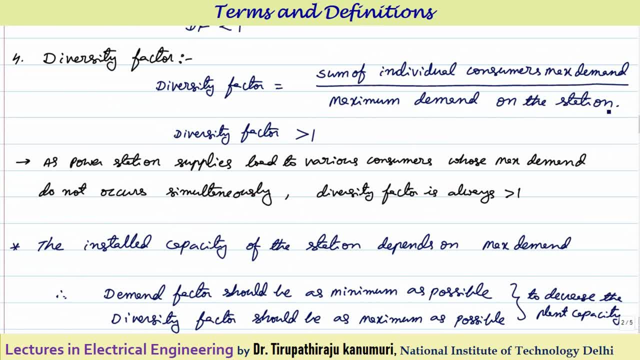 maximum demand on the station. Again, to explain this also, let us take, for example, there is a substation, So that substation is connected to different houses, So different consumers will consume or take the maximum demand at different timings, So like different people will have the 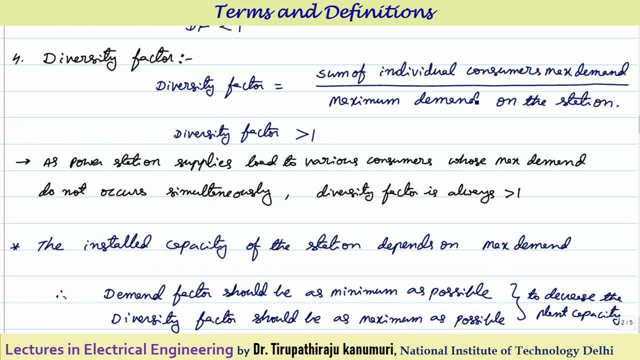 demand at different timings. Let us take, for example, if you take on a power station, that power station is supplying different type of power, So that power station is supplying different type of consumers, Like it is supplying the household consumers. Generally, household consumers consume the. 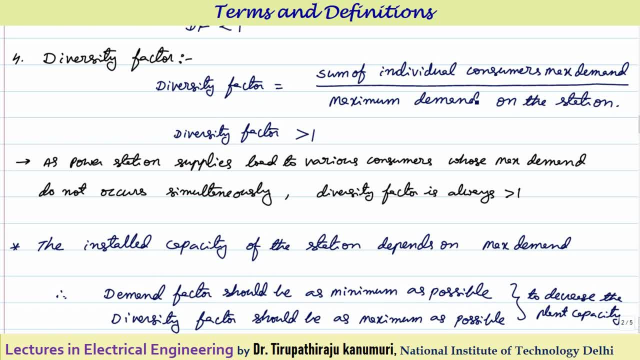 maximum power in the morning where they are getting ready for their office. Again, they will consume the maximum power between 6 to 9 in the evening. So remaining timings that demand will be very less. That means maximum demand happens for the consumers- household consumers- in the morning and evening. 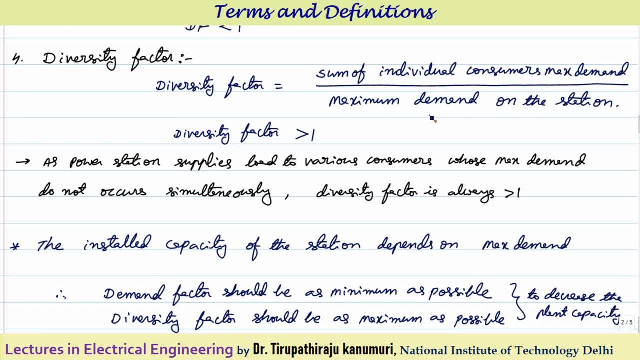 So let us take for example, there is a industry also connected to that power station. So industries, generally they open at 9 o'clock and they will run up to 6 or 7 o'clock in the evening. Generally they run up to 7 or 8 o'clock in the evening and very few industries run for the 24 hours. So there is another type of 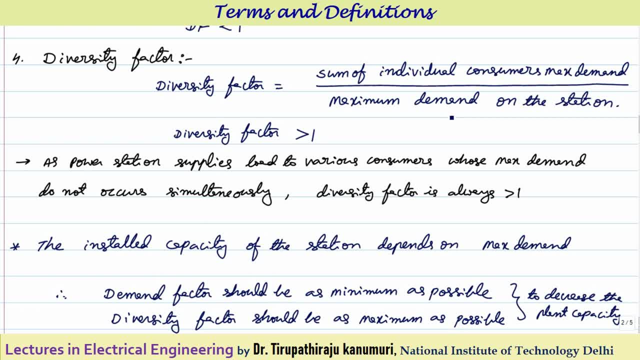 loads called as commercial loads. Commercial load means if you take the shops or other things, Generally the shops also. they open by 11 o'clock, then close by 7 or 8 o'clock, So their maximum demand is during that time only. That means we can tell that the maximum demands occurs at different. 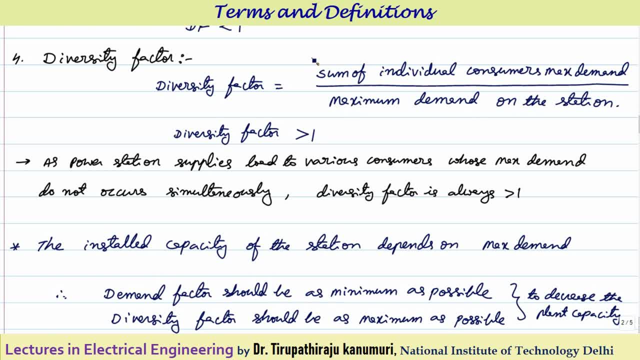 instances for different type of consumers. That's why always the maximum demand on the station will be less than some of the individual maximum demands of the consumers. That means we can tell that always the diversity factor will be greater than one. always the diversity factor will. 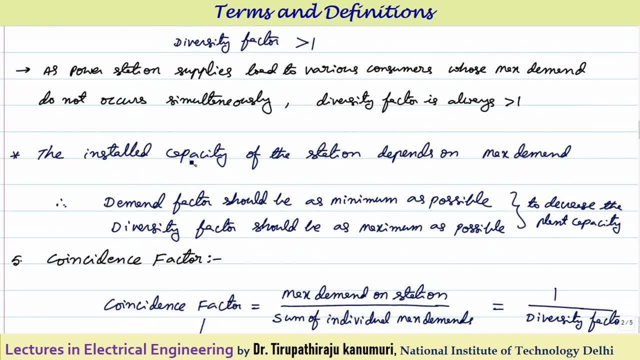 be greater than one. so let us try to make the conclusion up to here, then we'll proceed further. so always, the installed capacity of a station mainly depends on the overall maximum demand on the power station. that means always your power station should be capable of supplying this. 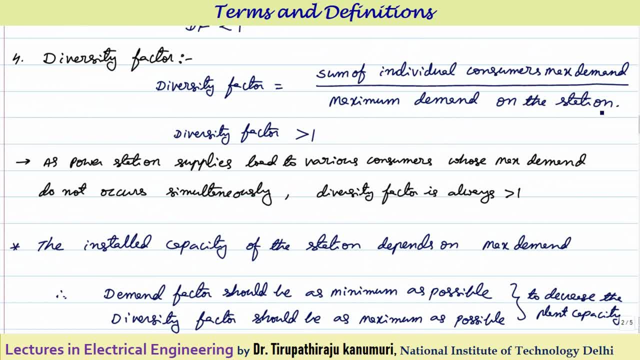 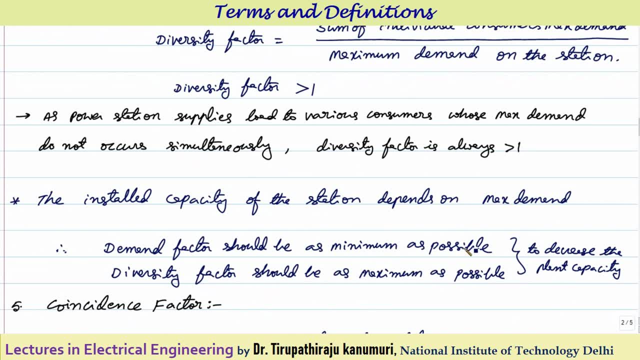 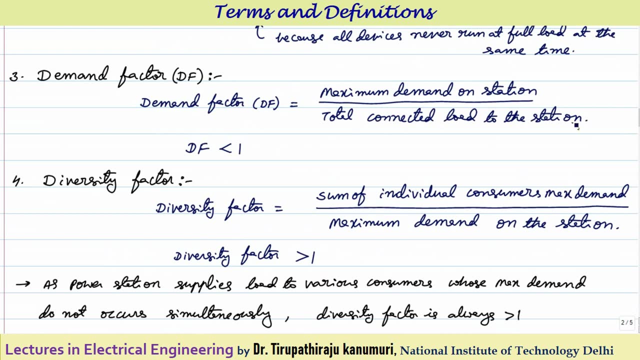 maximum demand on the station. that means simultaneous maximum demand on the station. accordingly the installed capacity is decided. so we can tell that the demand factor should be as minimum as possible. so what is the demand factor? demand factor is maximum demand on the station by total connected load on the station. even though the connected load on the station 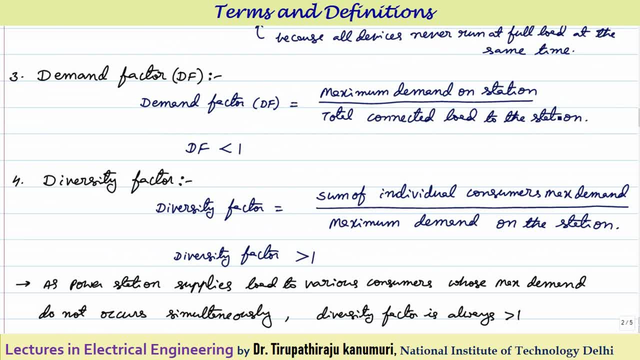 may be more if the maximum demand is less, automatically in order to supply the given connected load. so the power plant capacity is decreased, so automatically initial investment decreases. so i want that my demand factor should be as less as possible. so now coming to the diversity factor, so the sum of individual consumers, maximum demand, divided by 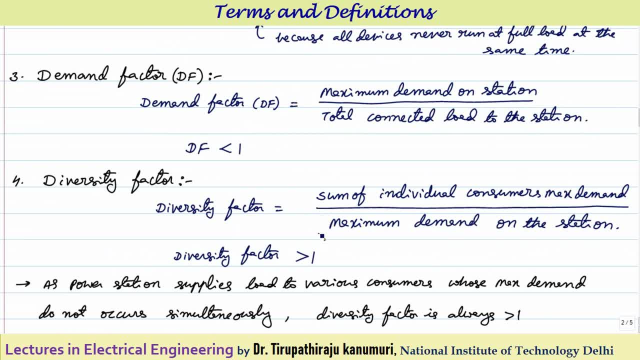 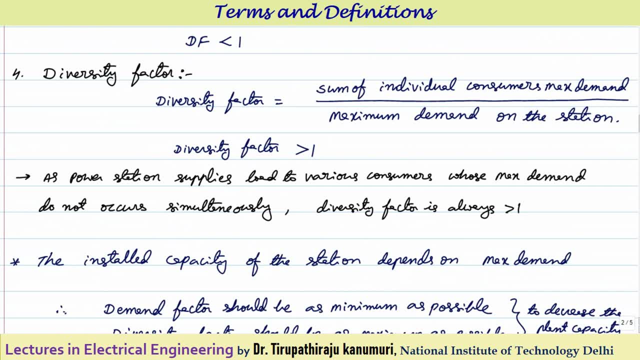 maximum demand on the station. i want my maximum demand on the station should be minimum, so so i want my diversity factor should be as maximum as possible. so more the diversity factor, i can tell that lesser will be the capacity of the plant required in order to supply the respective 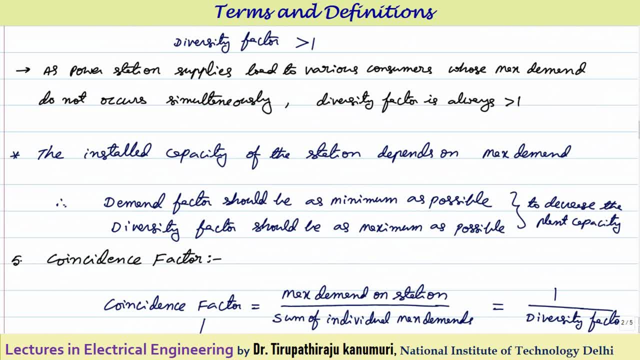 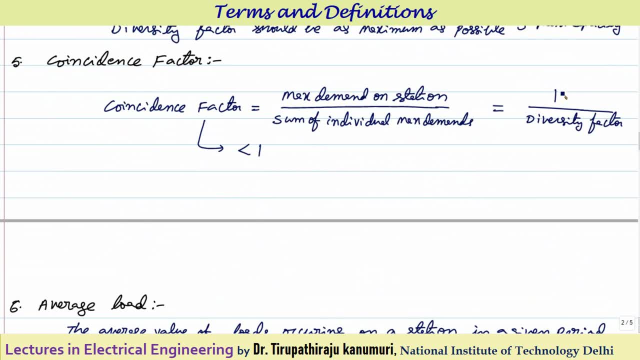 maximum demands, so lesser will be the cost per unit that is generated. so then comes another factor that is also called as coincidence factor. so this coincidence factor is the reciprocal of the diversity factor. that means it is a ratio of maximum demand on the station divided by sum of individual markets and demands. this will be less than one. so then comes the average load. 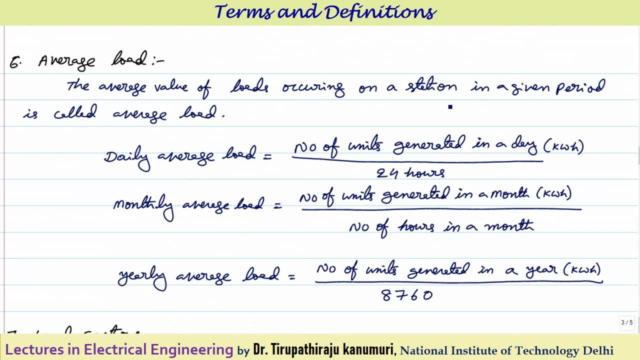 the average load is the average value of the loads occurring on a station in a given period that is called as the average road. this average load can be either daily average load, monthly average load or yearly average load. it means that days avoidanceキUE is equal to the average load. if the average load is negative, then the average load or progression load is notowy average load. if 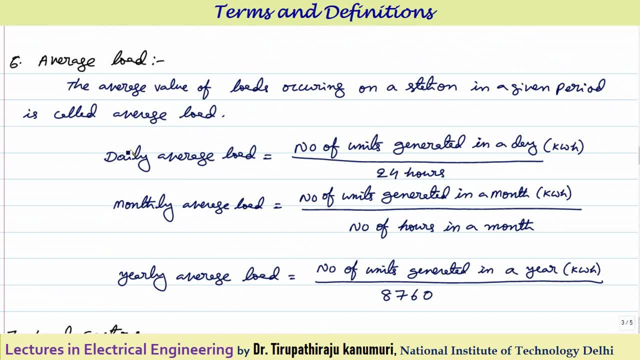 road. it depends on how many hours we are counting. so let us take, for example, diary. average road will be number of units generated in a day. that will be represented in kilowatt hour divided by total, total number of hours in a day, because this load will be in kilowatt. so kilowatt hour divided by 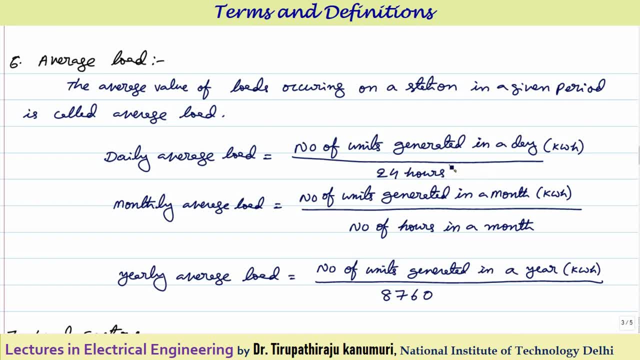 hours, so per day there are 24 hours. you have to divide by 24. similarly, monthly average road means number of units generated in a month divided by number of hours in a month. i have not mentioned the number here because number of days can be 28, 30 or 31 for different different months. so then, 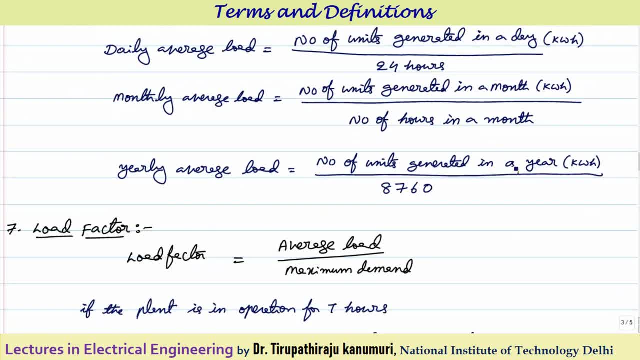 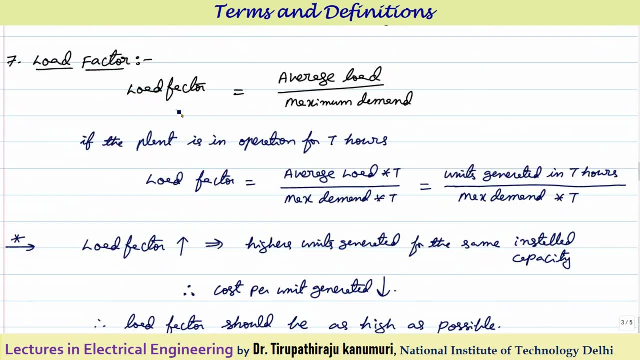 coming to yearly average road will be equal to number of units generated in a year in kilowatt hour divided by because we know there will be generally 365 days. so that will be equal to 365 multiplied by 24. you will get it as 8740 hours. then comes the load factor, so load factor is a 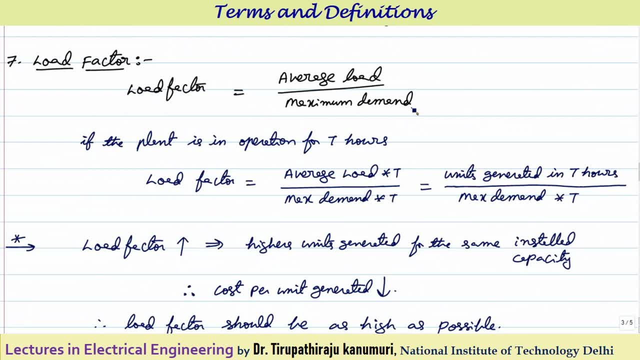 ratio of average load divided by maximum demand. this is the average load divided by maximum demand. so what i am doing, i am multiplying both numerator and denominator with the time t. t is the number of hours per with your plant is in operation. so average load multiplied by the time, so that gives, because average load is a total units. 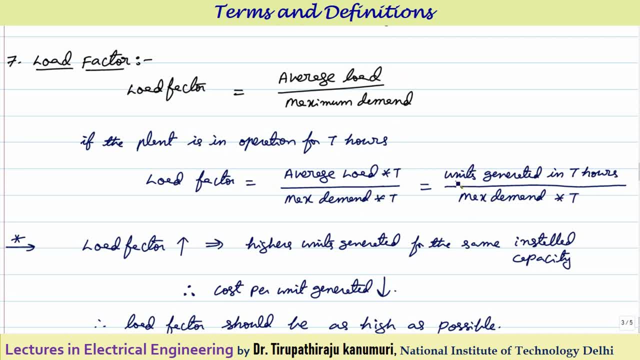 generated divided by time. so you are multiplying with time, so that gives total number of units generated in this t hours divided by maximum demand into time. so this is this in this way also i can define, so you can observe here: so as a demand factor is increasing as a demand factor. 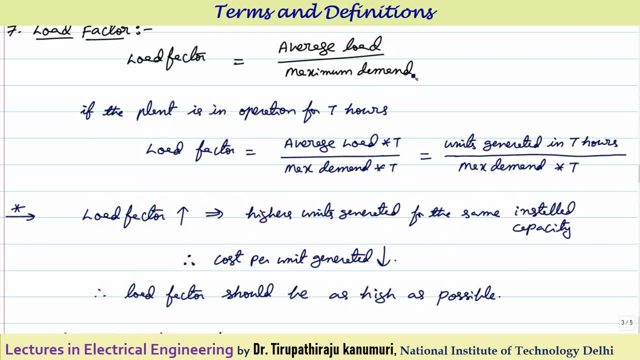 is increasing. what is the meaning of that? for a given maximum demand, the average load is increasing. so we know that the plant install capacity depends on the maximum demand. so for a given install capacity of the plant, more the average load, that means more power is generated. that 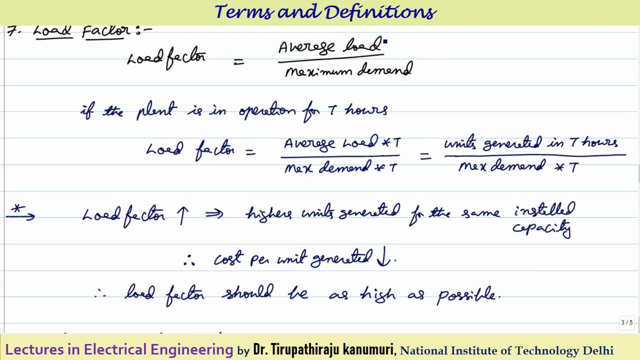 means more the income is generated for our plant. so that's why we can supply at a lesser cost per unit, because for a given investment, because the initial or the huge investment for any power plant will be the purchase of all the generator or the installed capacity, only the running cost will be less main. 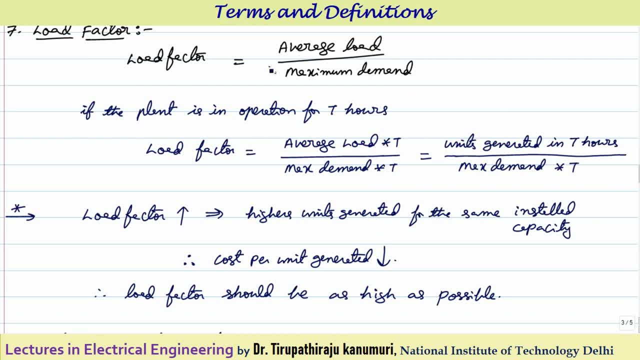 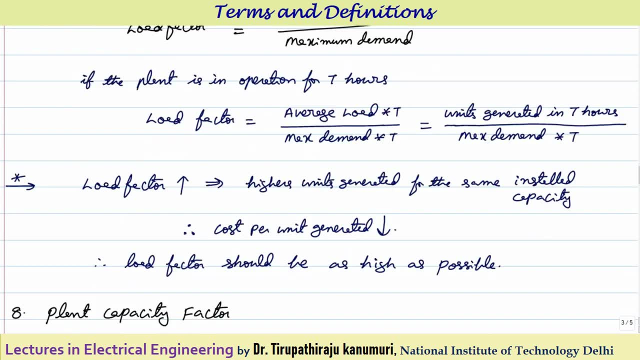 thing will be that initial cost will be very huge. so if the maximum demand is less, so automatically the initial investment is less, so we can supply at a lesser rate per unit. so the same thing i have explained here: as the power factor increased, higher units are generated for the same installed. 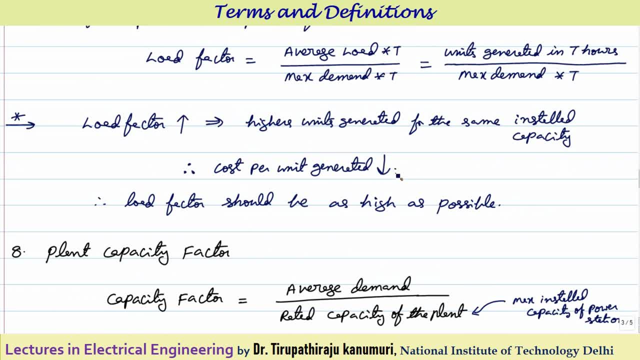 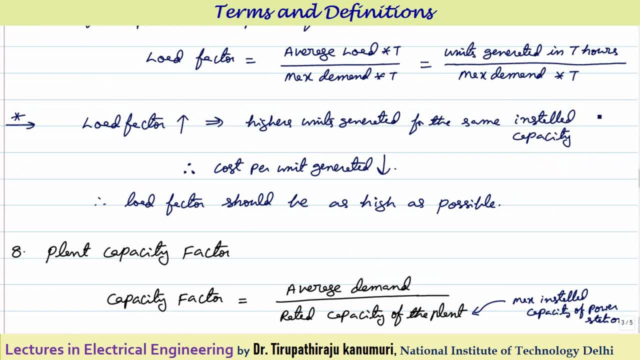 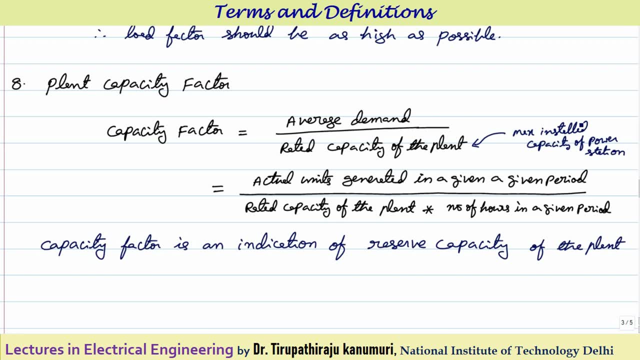 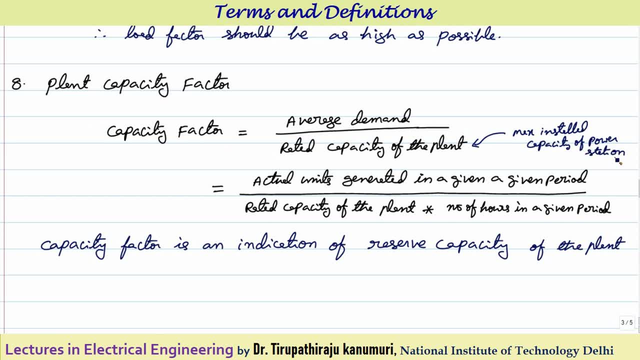 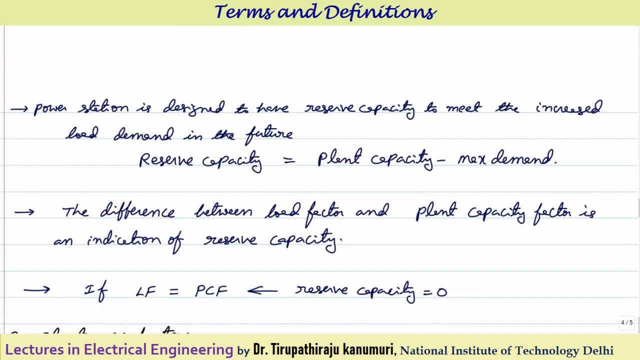 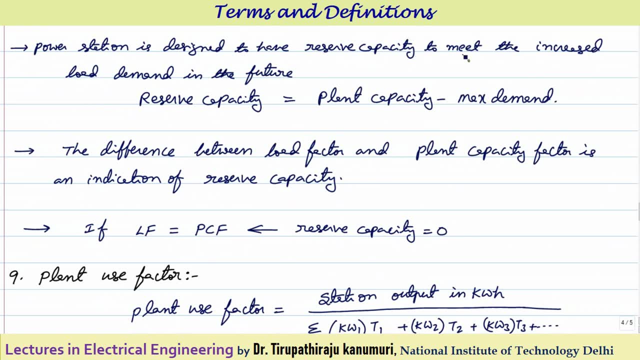 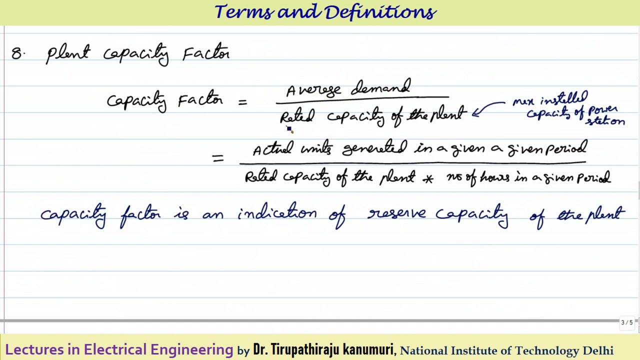 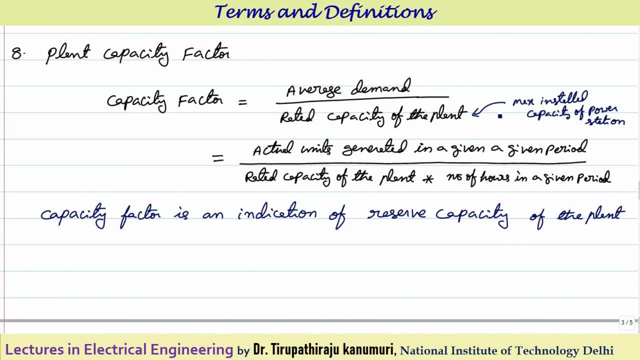 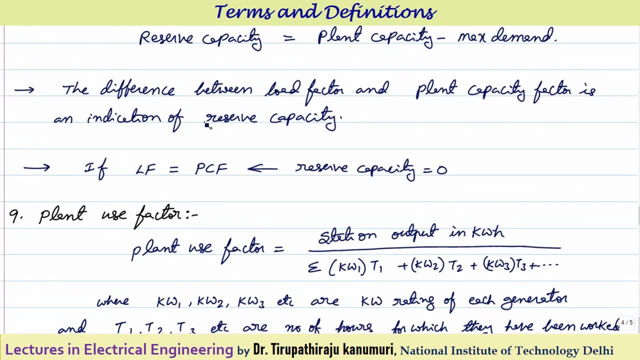 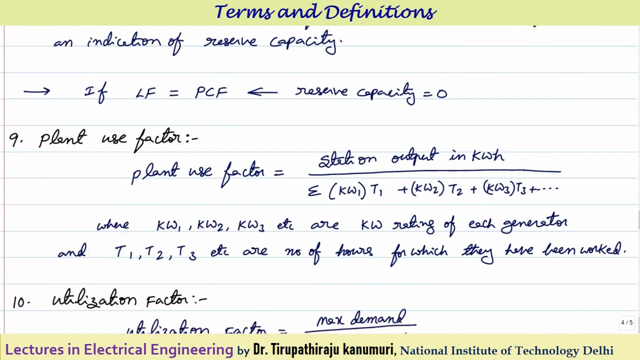 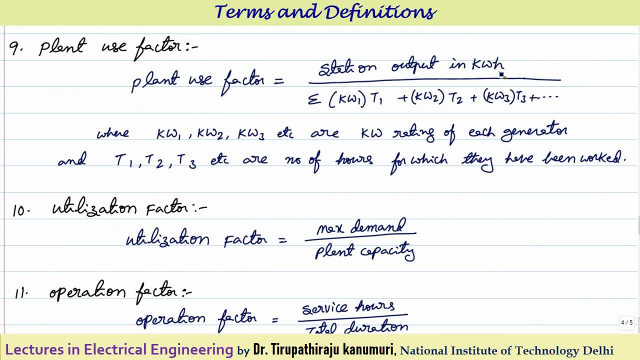 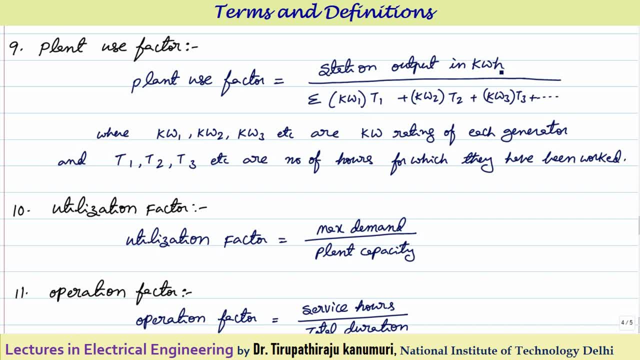 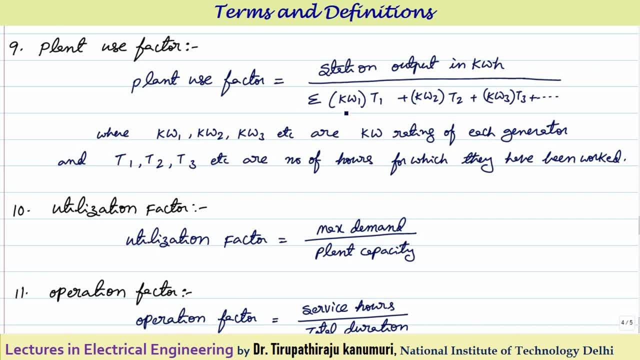 efficiency of your plant. thereby we can supply at a lesser cost per unit. so that's why- let i assume my power plant is having different rating of the units that i am representing by first generator is having kw1, second generator kw2, third generator kwt. and let i assume the first generator is: 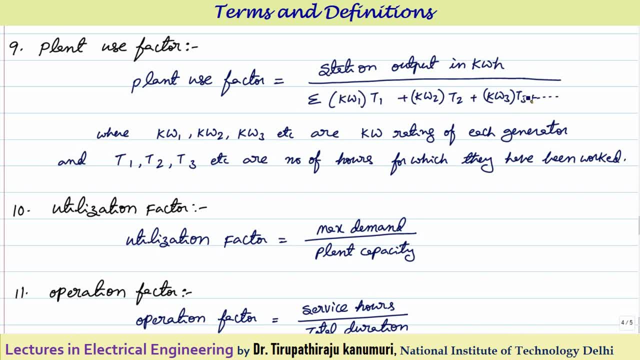 running for a time t1. second generator is running for a time t2. third generator is running for a time t3, and so on. so if you want to calculate the plant use factor, plant use factor will be equal to station output in kilowatt hour divided by sum of all these things. so you have to take 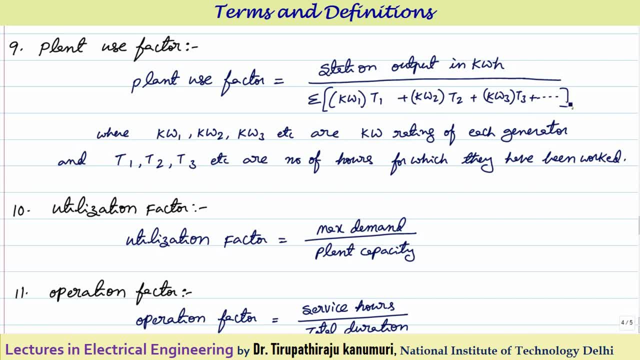 the sum of kw1, t1 plus kw2, t2 plus, etc. all these things. so this indicates the plant use factor getting it. so the difference between plant use factor and the plant capacity factor is, in the previous case, what we are doing. we are just multiplying the plant capacity with the 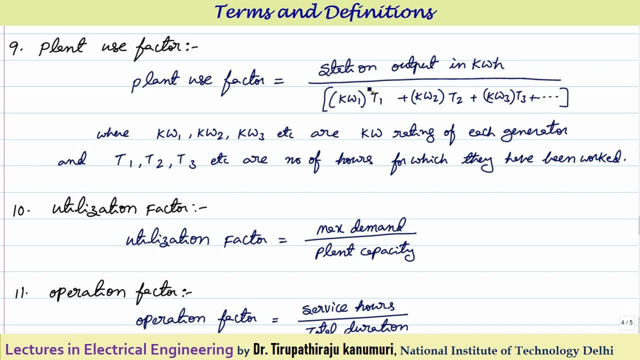 two units. so we are multiplying the plant capacity with the two units, so we are multiplying the plant total time of operation. but here, because we know all the units are not operating throughout the time. so that's why here we are considering the actual time of operation, so this is more practical. 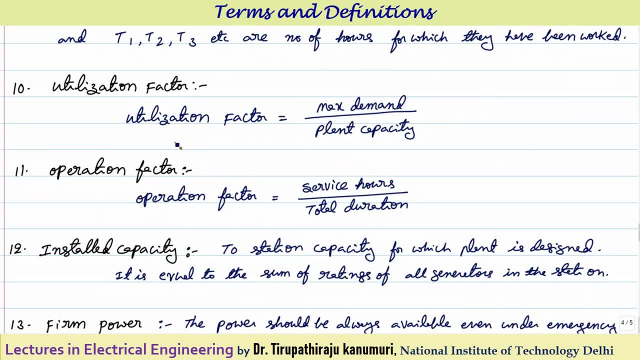 than the previous one. so then comes the utilization factor. the utilization factor is a ratio of maximum demand divided by plant capacity. maximum demand divided by plant capacity. out of the installed capacity, how much is actually supplied because remaining things remains as not useful? actually, they are purchased for the future purpose but not in use now. then comes the. 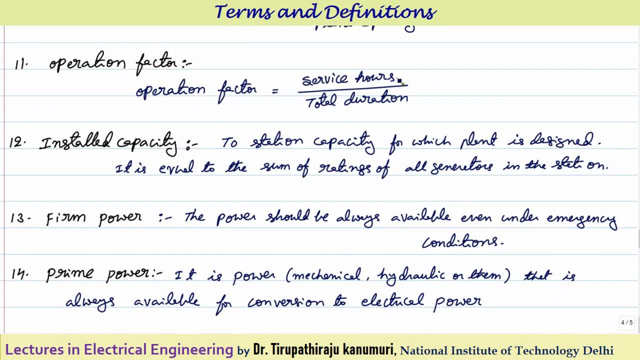 operation factor. the operation factor is a ratio of service hours divided by total duration. like, for example, your power plant is working for 300 year, 300 hours or 300 days out of the 365 days, so operation factor will be 300 divided by 365. so in that way we can calculate, or if it is operation. 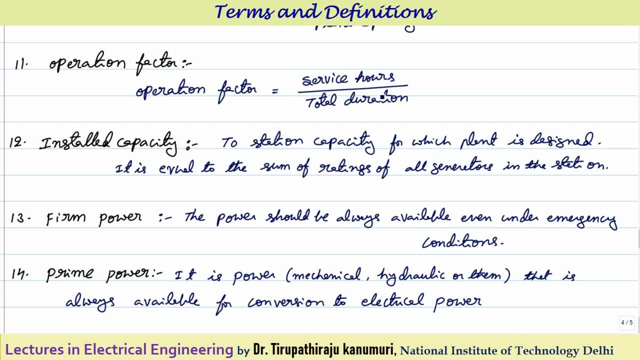 for particular hours of the year. so number of hours for which it is in operation, number of hours for which it is in operation divided by total number of hours in an year. in that way you can calculate. then comes the installed capacity. the name itself is telling to. it is the station capacity for which the 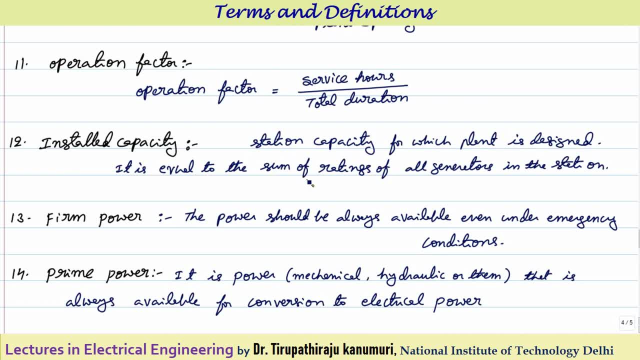 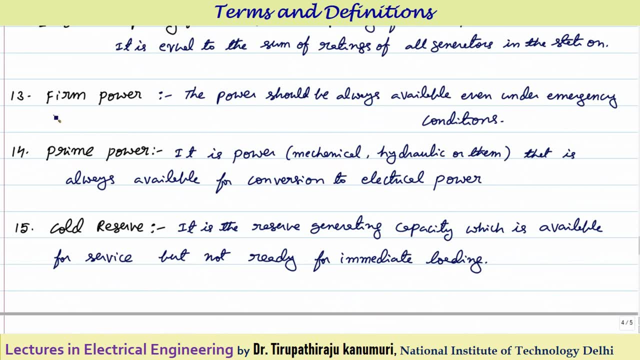 plant is designed or it is nothing. but it is equal to the sum of a rating of all the generators in the station, so that is called as the installed capacity. so then comes the firm power, the power which should always be available, even under the emergency conditions. that is called as the firm. 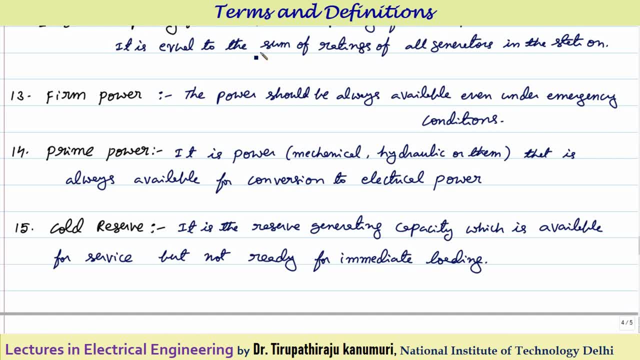 power. that means out of the entire power generated by the power plant. we will design in such a way that some power can be generated even under emergency condition. that is called as a firm power. then comes the prime power. prime power is it is a power, that power can be either mechanical. 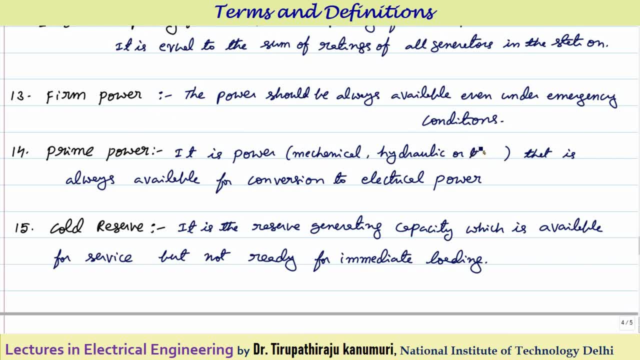 hydraulic or thermal. this can be hydraulic or thermal. that is always available for conversion to electrical power too. that means we can tell that the prime power is nothing, but because we know the generator is is run by a prime mover. so the power that is available at the prime over that is called as a 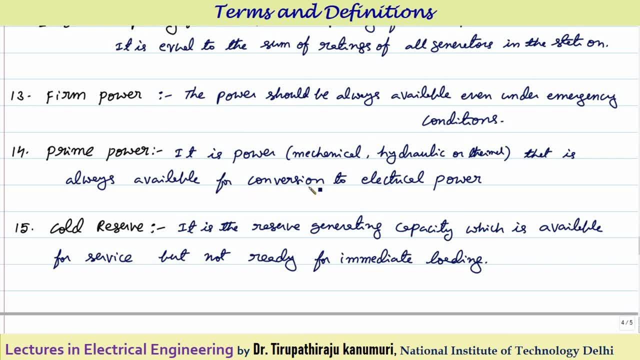 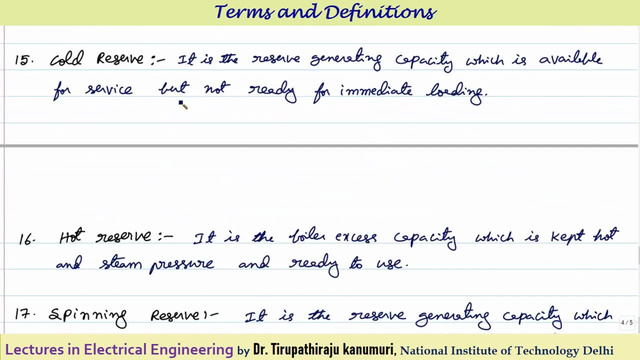 prime power. that means it is a power, because that can be either mechanical power, hydraulic power or even it can be thermal power that is always available for conversion. so then comes the cold reserve and hot reserve and spinning reserve. again, these three are also generally confusing topics. so 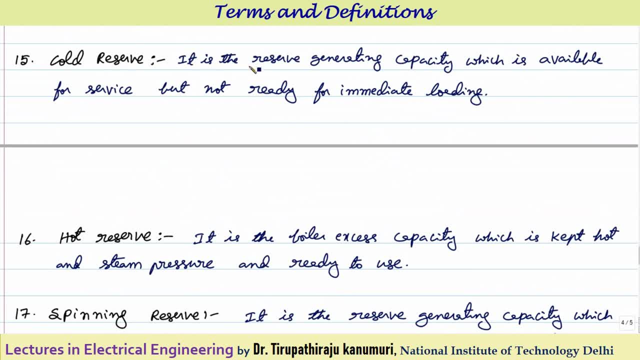 let us discuss them first. one is the cold reserve. then name itself helps in the situation of' self-installing cold. so what does it mean? it is a reserve generating capacity which is available for service but not ready for immediate loading. so i am reading once again: it is a reserve. 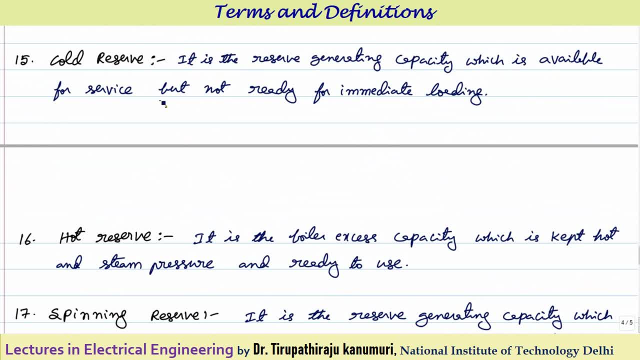 generating capacity which is available for service but not ready for the immediate loading. let us assume i am having a power plant where it is having some 100 kilowatt generators. of five generators out of five generators, let us assume four generators are running and one generator is shut down. one generator is not running now. so if the generator actually it is, 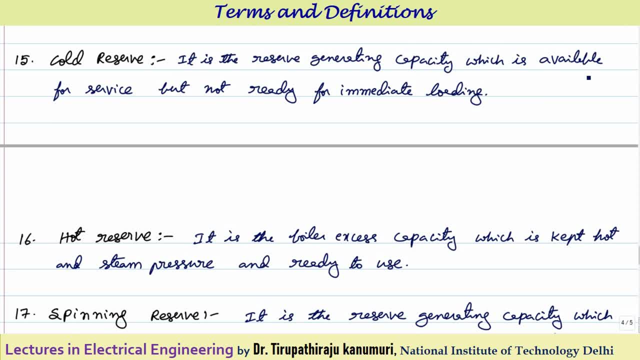 one working condition only, but cannot be operated immediately, because if you want to operate the generator, what you have to do you have to turn on the generator by supplying the steam input, then synchronize to the grid, then only it will start supplying to the grid, actually the generator. 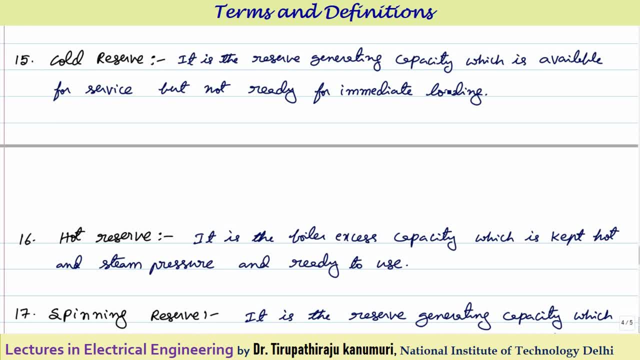 is. it is an operating condition but currently not working, so that is called as the cold reserve. then comes the hot reserve. hot reserve means it is the boiler excess capacity which is kept hot and steam pressure and ready to use. that means cold reserve means it is not ready to use, hot reserve means it is. 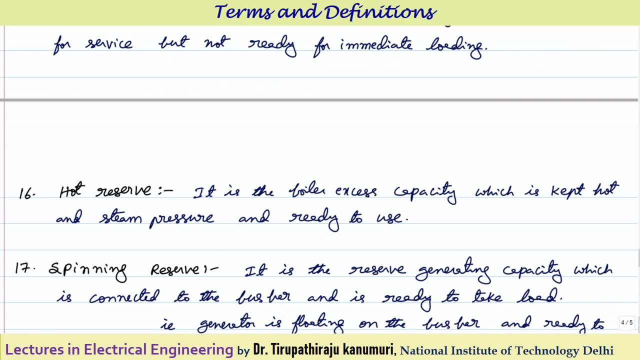 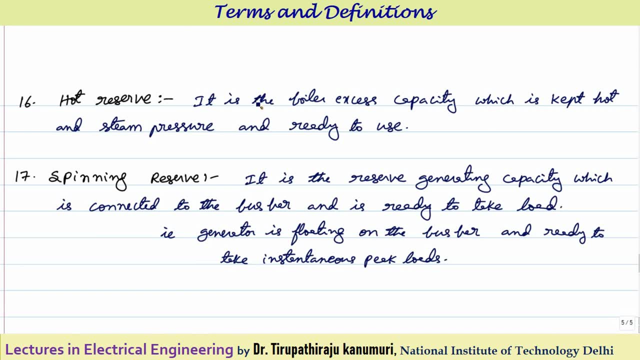 ready to use. that means we can use it readily. that means the steam is ready and we can supply the steam and start producing the power that is called as hot reserve. again this one also. actually it is not supplying. it is ready to supply, but it is not actually supplying. then comes another. 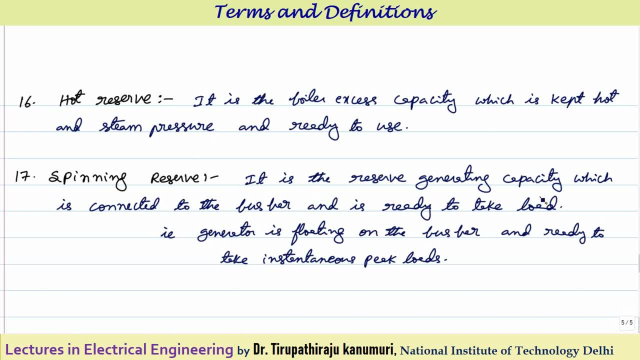 term called as the spinning reserve. so it is a reserve generating capacity which is connected to the bus bar and is ready to take the load, which is connected to the bus bar and ready to take the load. so what is the meaning of this one? so in this case, the generator is already started and 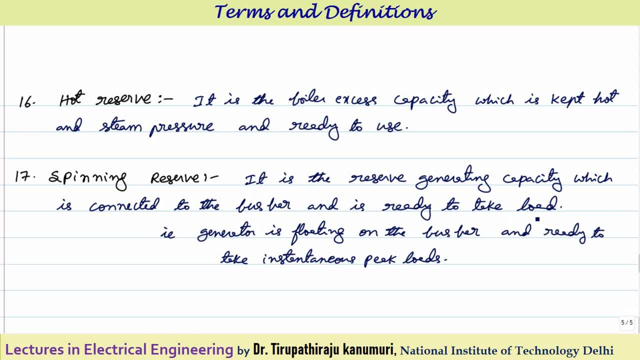 synchronized to the grid also, and the steam input and everything is already given to the generator. but that generator is not supplying the load. but the generator is not supplying the load, waiting for the load to increase so that it can share the load. I am repeating once again these three. 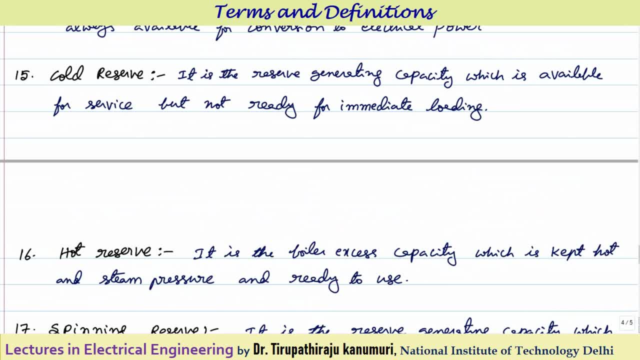 reserves. cold reserve means there is a generator which is in the working condition but currently not working. I am repeating once again: there is a generator which is not started or connected to the grid. that is called as the cold reserve. then comes the hot reserve. hot reserve means that 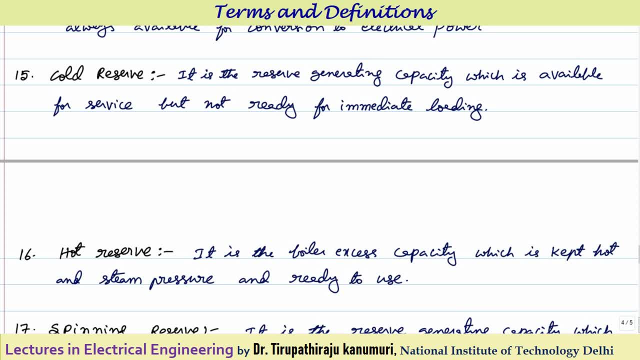 generator because the steam, input and everything is already readily available. that means we can make it run and connect to the grid again. in the case of hot reserve, it is not connected to the grid, but the generator is ready to operate. you have to give the steam and 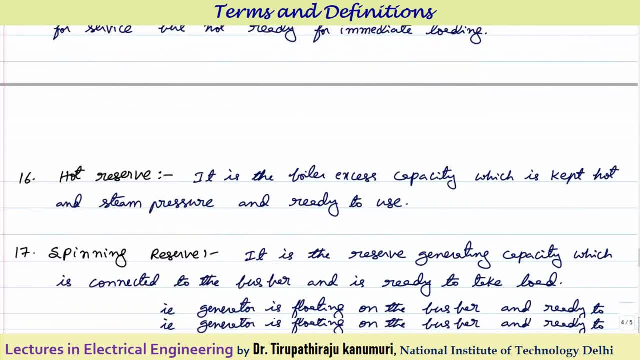 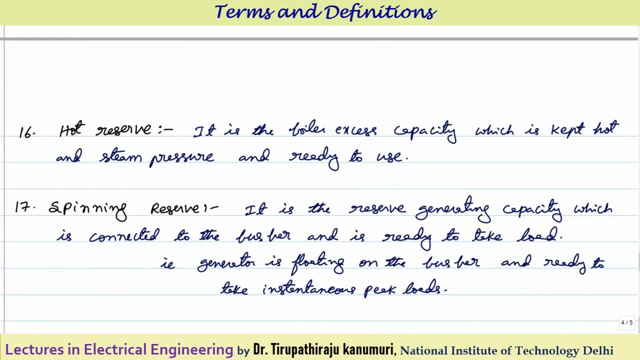 just synchronize to the supply, then it will start working. then comes the spinning reserve. spinning reserve means the generator is operating and the steam input is also given. it is connected to grid also, but actually it is ready to supply the load just by increasing the loading automatically. it. 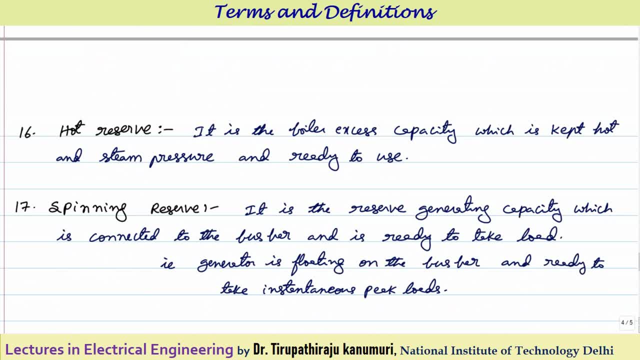 will start supplying. that means the generator is ready to supply the extra load. so the spinning reserve term is generally used. the generator is putting on the bus bar and ready to take the instantaneous peak loads. it is ready to take the instantaneous peak loads. that is called a spinning reserve. I hope all the terms related to economics. 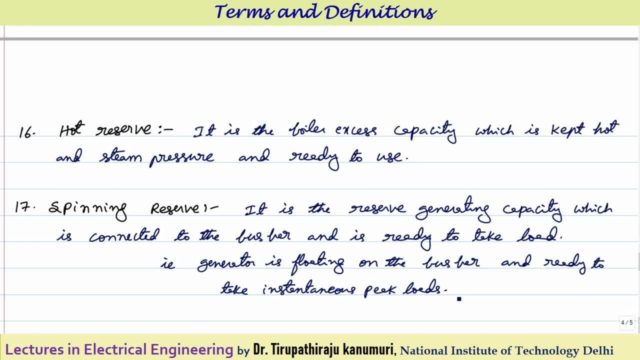 are completely clear to you. if you still have any queries, you can leave your comments in the comment section below. I will answer to your queries from there, thank you. thank you very much.